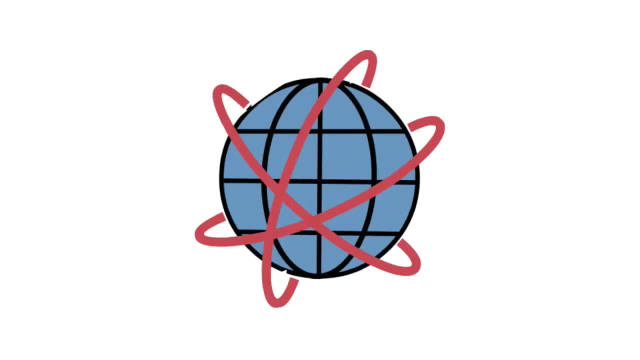 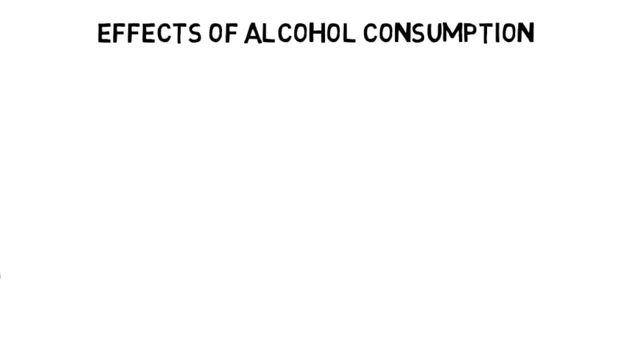 Alcohol consumption has become socially acceptable for adolescents as a means of self-exploration and transition. However, many short-term and long-term side effects exist with various levels of consumption. Immediate implications of alcohol consumption include slurred speech, drowsiness, vomiting. 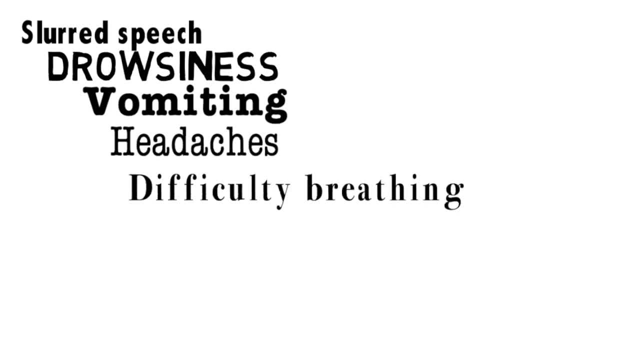 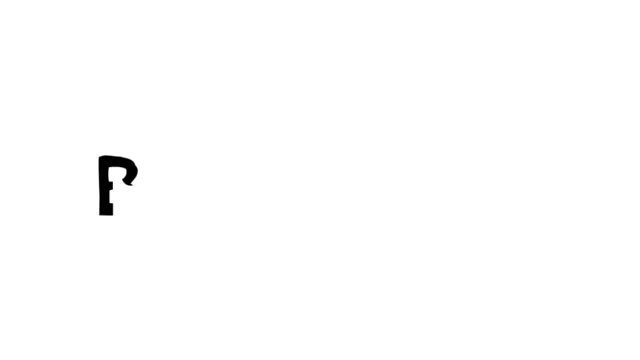 headaches, difficulty breathing, distorted vision and hearing, impaired judgment, decreased perception and coordination and possible blackouts, or a person experiences memory lapse and doesn't remember events while under the influence of alcohol. There are several long-term effects of heavy consumption, including various cancers, alcohol-related. 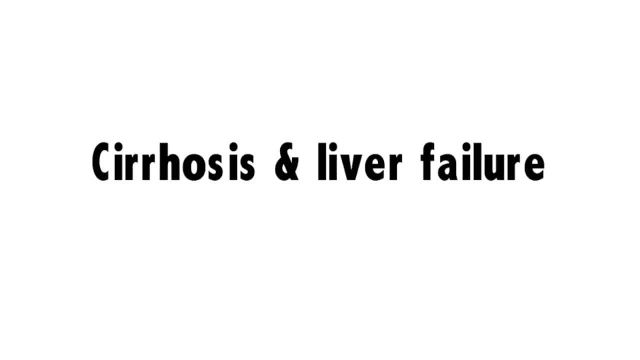 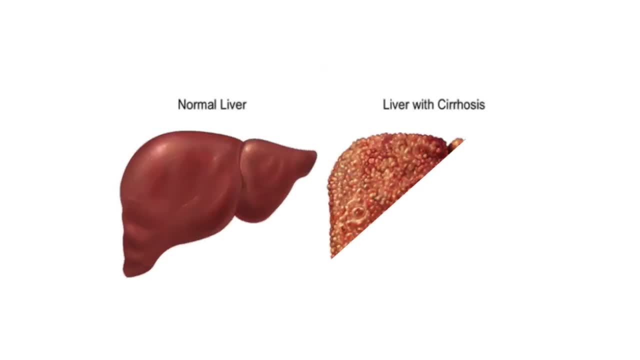 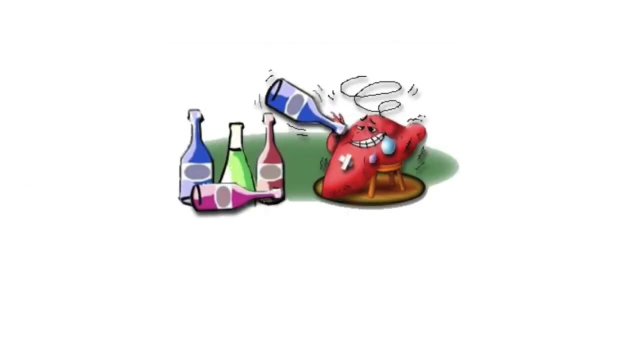 disease, hypertension and stroke. The most predominant long-term effect of alcohol consumption is cirrhosis and liver failure. Cirrhosis is a condition that develops when scarred tissue replaces healthy tissue of the liver. It occurs when healthy cells of the liver are constantly damaged over a period. 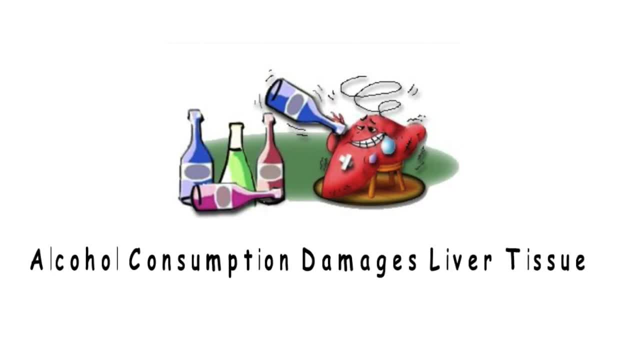 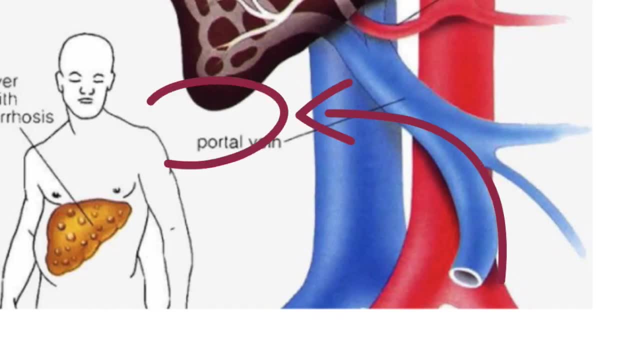 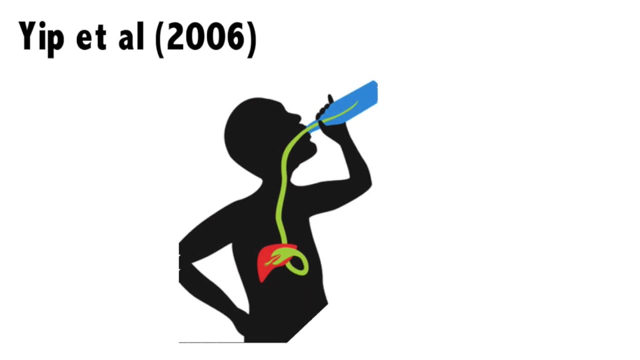 of time, usually many years, because of alcohol consumption. As a result, scarred liver tissue becomes hardened and lumpy and prevents the flow of blood through the large vein, known as the portal vein, into the liver. Hippe et al outlined how excessive alcohol consumption can lead to the cirrhosis of the liver. 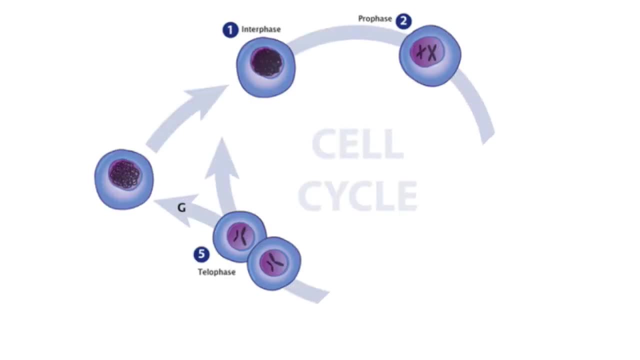 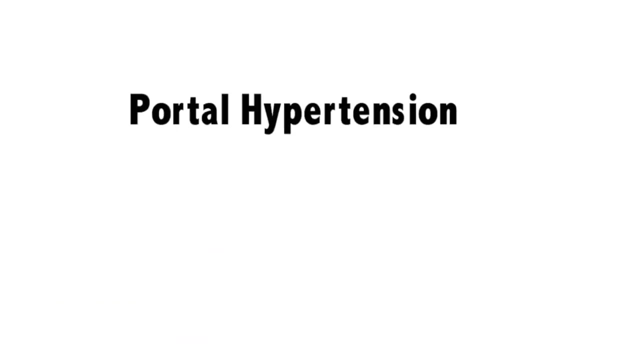 Over time, nodules fail to form due to the impaired division of cells in the liver. This consequently leads to distortion of the liver and the presence of portal hypertension, which is increased blood pressure within a system of the veins. Due to lack of cell division and the constant process of cell death, there is a drastic reduction in liver cells. 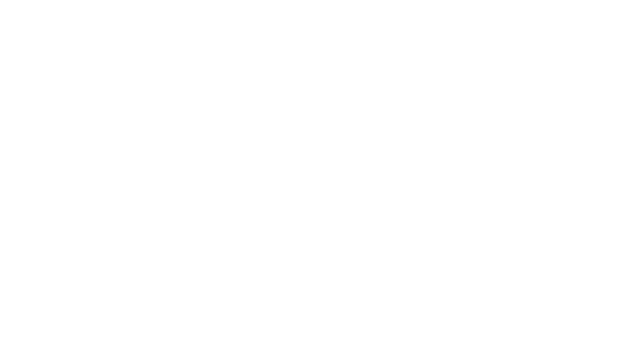 As a result, liver cirrhosis is established and can further lead to complete failure of the organ. Other evidence suggests a role of alcoholism in economic and social distress. Burke suggested that up to 50% of all emergency room admissions are alcohol-related. and healthcare costs for a family with an alcoholic member is twice as much as compared to one without Alcohol. consumption has been shown to be more prevalent among underaged individuals, especially in families where one or both parents are involved with excessive consumption. How can you identify if you or someone you know may have a drinking problem? 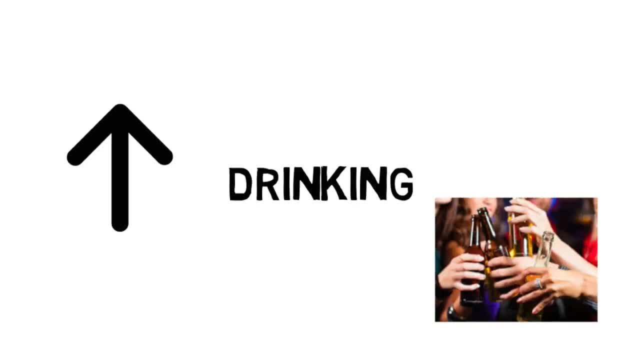 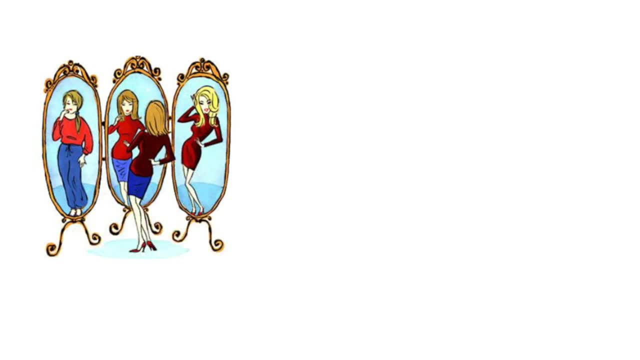 Some signs include an increase in the individual's drinking- drinking in the morning and drinking in non-social settings. There could also be changes in appearance, where a person constantly smells like alcohol, has slurred speech, bruises and possibly red eyes.